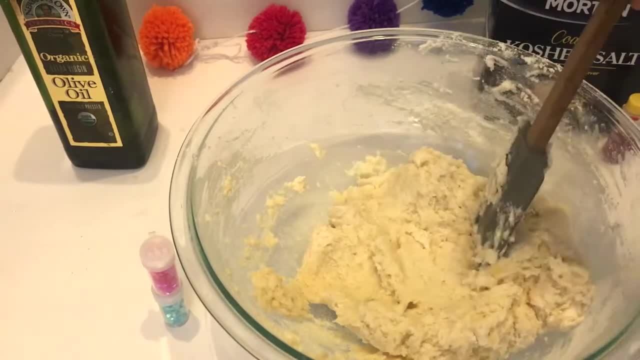 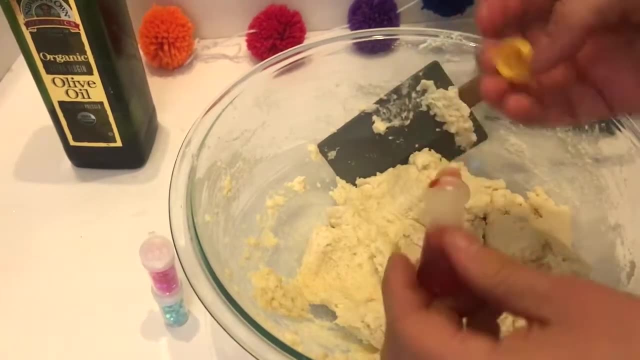 very hot. That's why we're using our spatula, and now we are going to add some other extra ingredients. So first we're going to try some food coloring. He chose yellow food coloring in, so we're just going to dump that in right away. 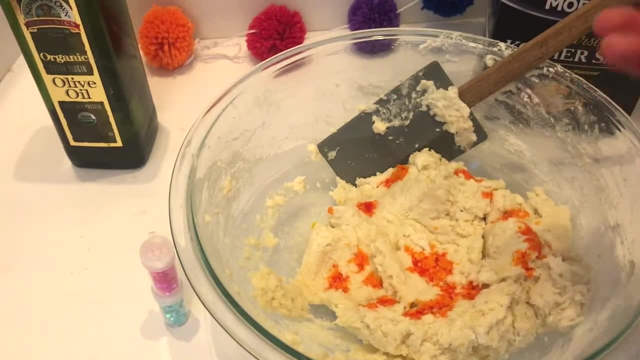 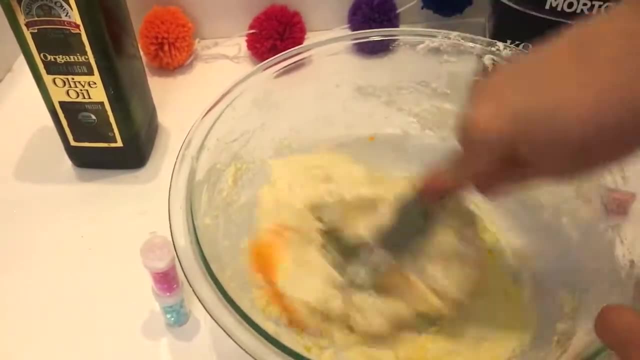 I think we'll put a lot in, because we want this to be really bright yellow. Then we're going to give it a mix here with our spatula, and if it's cold enough, you can just get right in there with your hands and mix it up and it will turn out really good. Okay, so we're mixing here, You can. 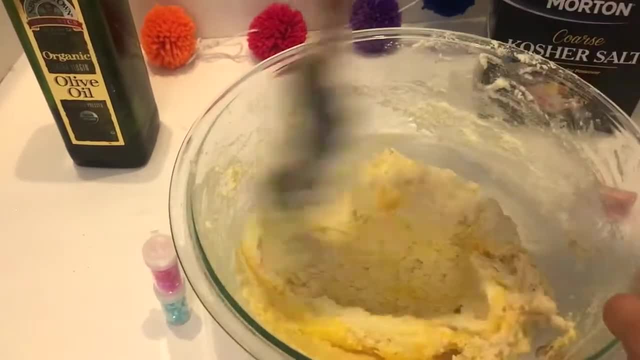 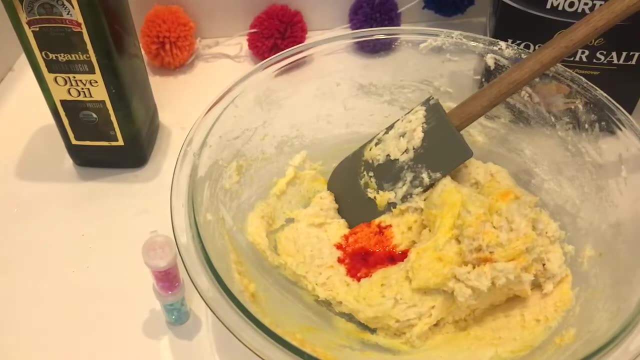 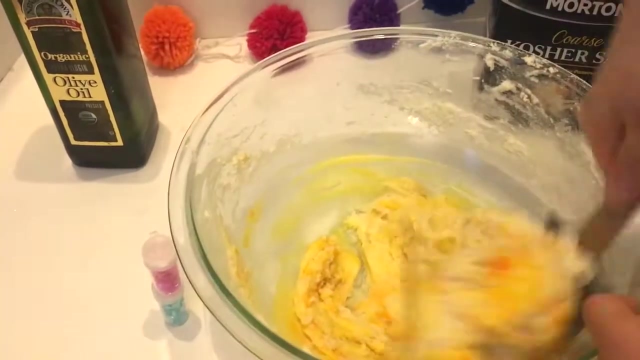 see that. you can see it turning yellow, and I think we might add just a little bit more food coloring, because we want this to be super bright. You can just kind of adjust to see how much food coloring you want. This is going to be super duper bright yellow. Okay, it's looking pretty good. I can still feel. 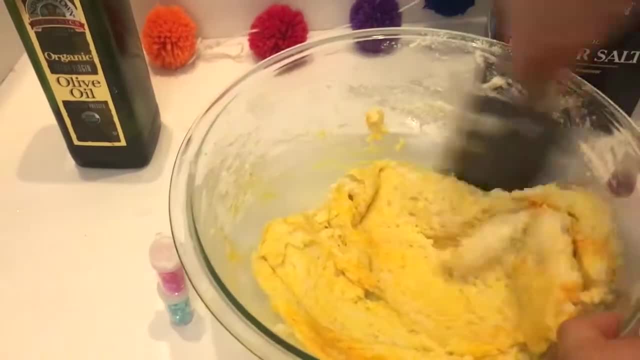 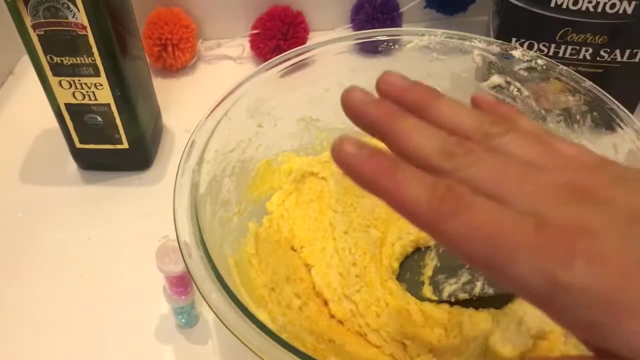 that it's very hot. So you want to make sure that you're going to do this with your, with your parents. Okay, look at it's turning. It's turning nice and bright yellow. So now we're going to add the fun part. We are going to add our sparkles to this Play-Doh. We've chosen sparkly pink, but I 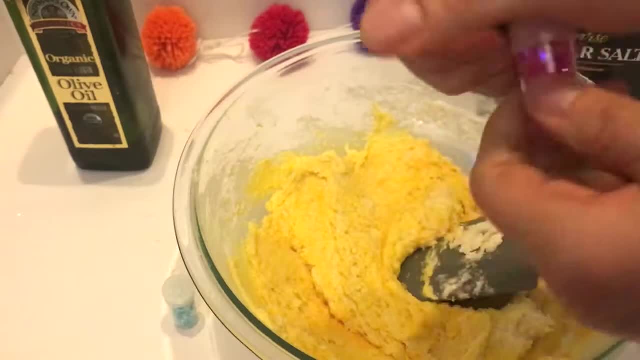 think we're just going to pop off the container because we want a lot of fun. So we're going to add the sparkles in here. So we're going to add our pink sparkles, Just dump it in, Whoa. okay, we've. 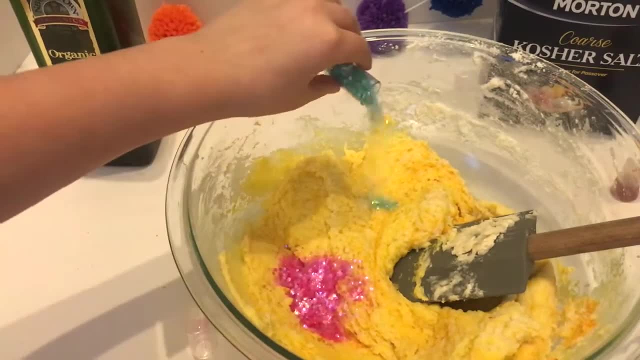 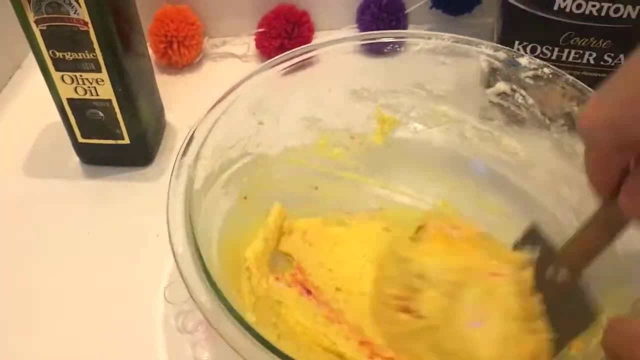 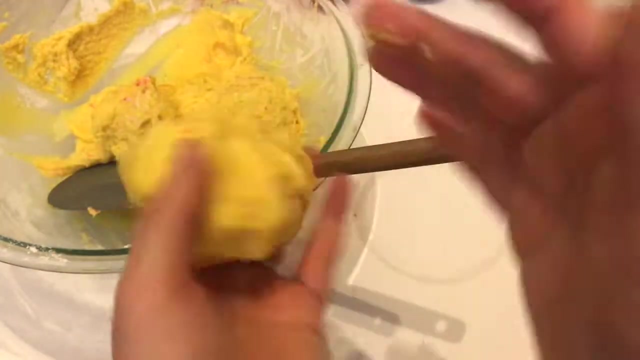 got pink in there, and now we're going to add our blue sparkles. Wow, look at that. Okay, now we're going to mix it again. Here we go, Okay, so this is the finished product, and once it cools down, you're going to be able to really mold it and shape it into whatever you want, As it's still. 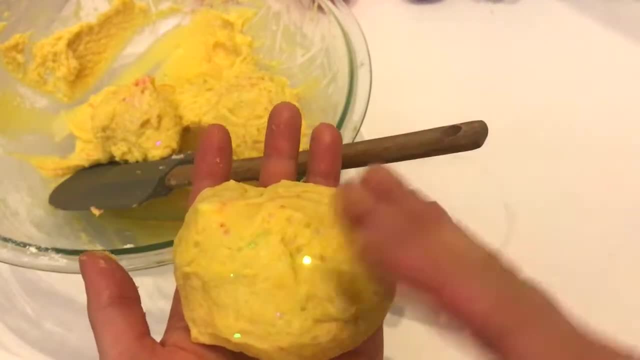 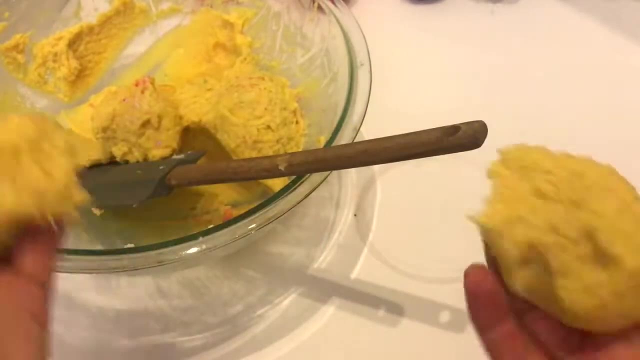 warm. it's still a little bit sticky and you can see my hands. I have a little bit of that Play-Doh stick on it but as soon as it cools down it's really ready to start playing with. and it is so soft and I really like this Play-Doh because it's really creamy and 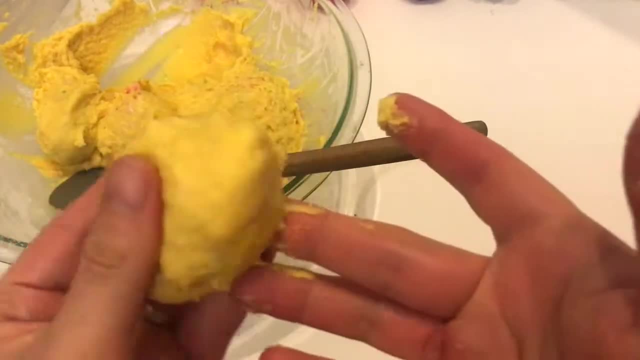 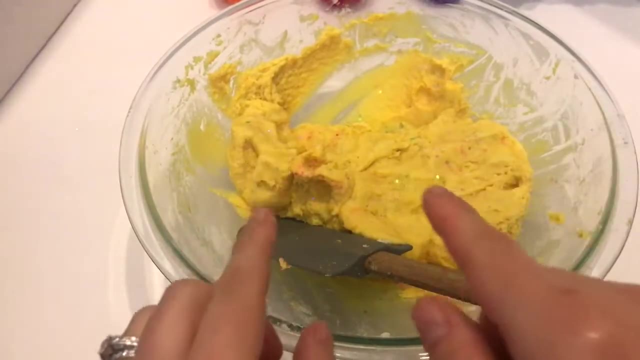 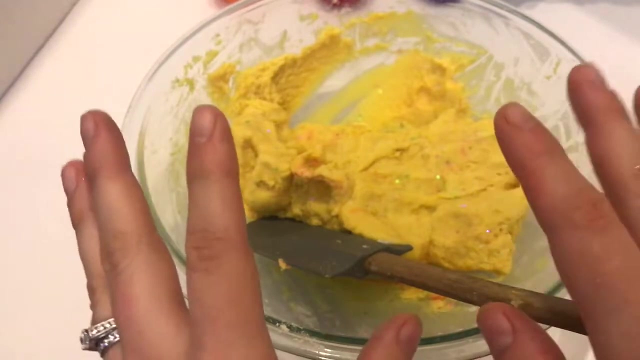 soft, It's not hard like some other Play-Dohs and it's just a really nice recipe. So if you like this video, give us a thumbs up, and if you made this Play-Doh and you love it, please leave us a comment down below. It is a really great Play-Doh and so I hope you liked it and subscribe.